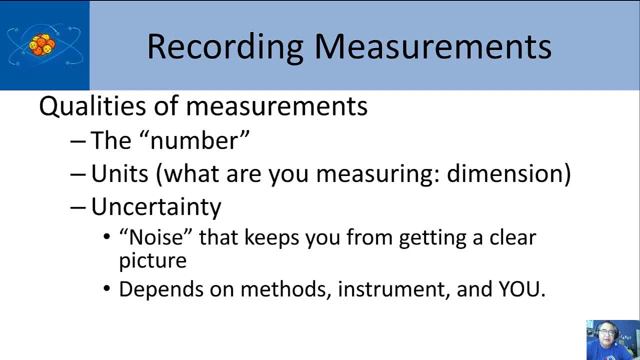 So you make a measurement right. Let's say, you put something on a balance, You'll get a number, for example, like 435.. But without the unit that's meaningless. So is that 435 grams or 435 pounds, or what kind of thing is it? 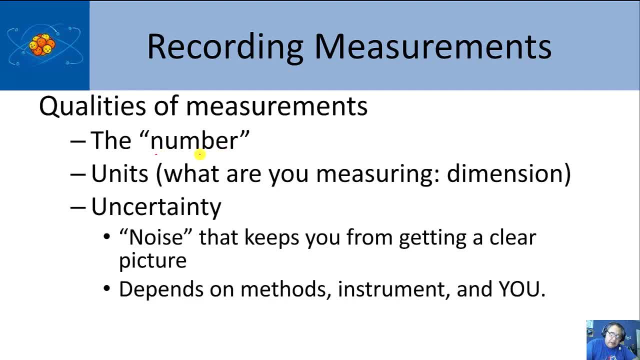 So we have a quantity, which is the number right, And then we have a unit, And then we have uncertainty. So if you take, let's say, you go to the grocery store, you know how, you have the old-fashioned pan balances that have a dial in it, right? 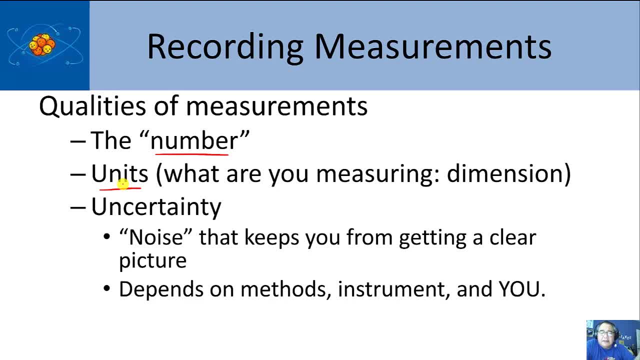 And you put food in there and you want to say, well, I need three pounds of fruit right Now. usually we're not that picky, But when you put it in there and you look at it, you know how the needle is like partway between two different numbers. 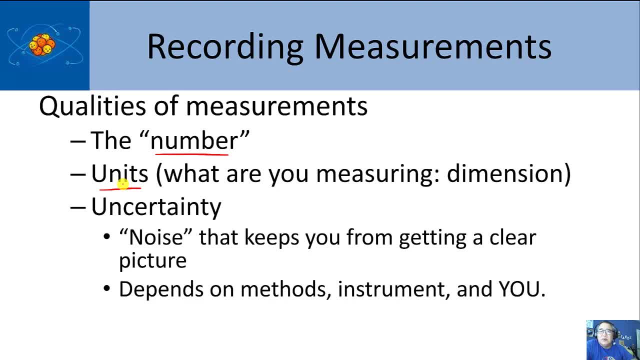 And so you have to try to guess, like: what does that number mean? So three pounds might be easy to see because of one, two and three. But what if you needed two and a half pounds? right, Then you'd have to sort of guess where the middle is. 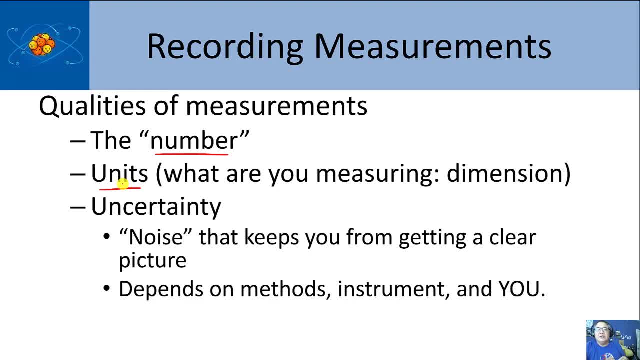 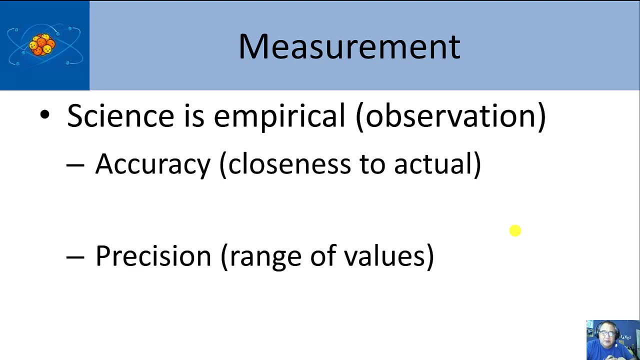 So we often refer to that as noise in the measurement or uncertainty in the measurement. We try to read it and get the right number. We're kind of guessing a little bit, And so significant figures will help us deal with that uncertainty. So science in general is empirical. 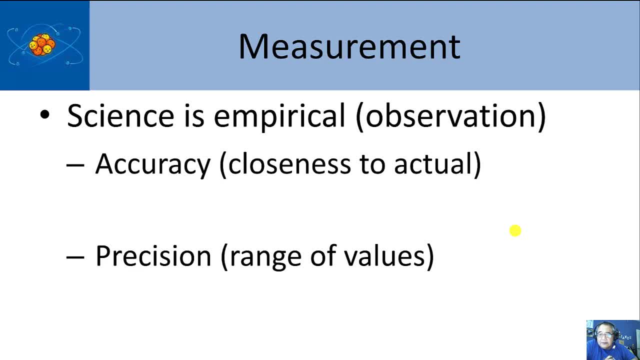 Chemistry, we say, is empirical science. There are also some theoretical sciences that are not based on observation, But an observation would be something like a measurement. okay, So accuracy is really what we refer to when a number is close to what the actual number is. 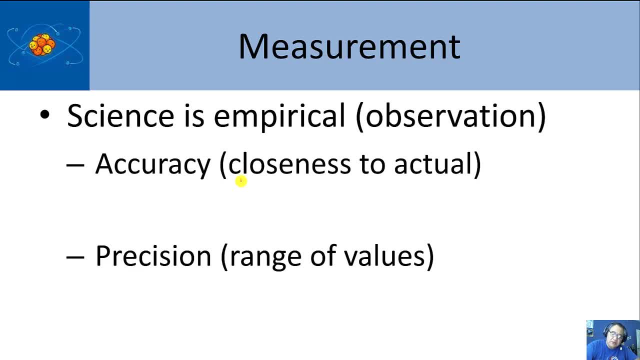 So the drawback to accuracy- right, This is closeness to the actual- The drawback to accuracy is that you may not know the actual number, And so you have to make a measurement and hope that it's accurate. But there's also another term and these two terms get mixed up in our language. okay, 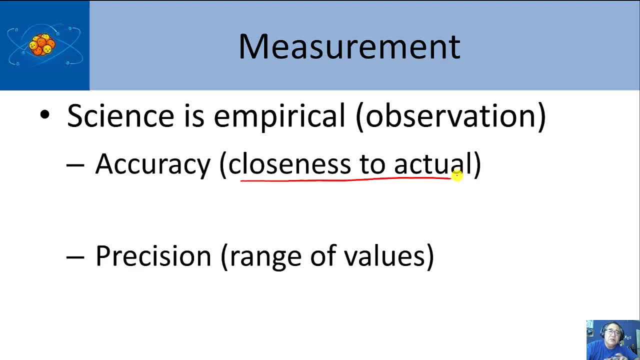 It's called precision And in general what's assumed in science is if your numbers are precise, then there's a good chance that you're going to get a good number. So if you're going to get a good number, then you're going to get a good number. 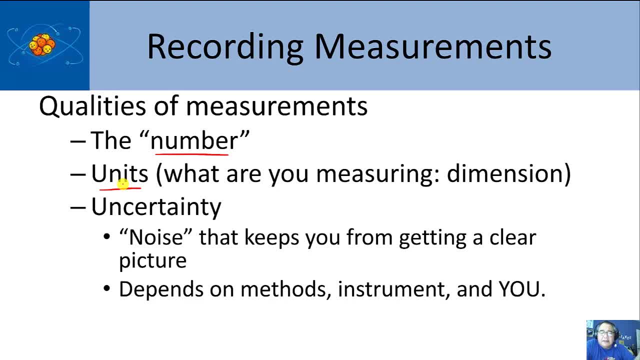 And you put food in there And you want to say, well, I need three pounds of fruit right Now. usually we're not that picky, But when you put it in there and you look at it, you know how the needle is like partway between two different numbers. 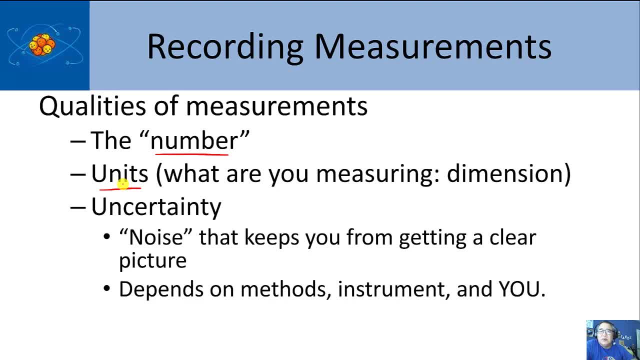 And so you have to try to guess, like: what does that number mean? So three pounds might be easy to see because of one, two and three. But what if you needed two and a half pounds? right, Then you'd have to sort of guess where the middle is. 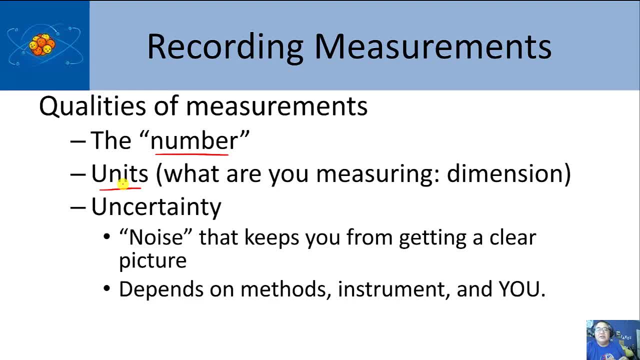 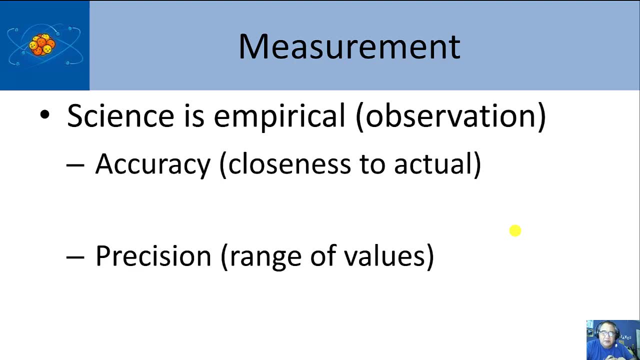 So we often refer to that as noise in the measurement or uncertainty in the measurement. We try to read it and get the right number, But we're kind of guessing a little bit, And so significant figures will help us deal with that uncertainty. So science in general is empirical. 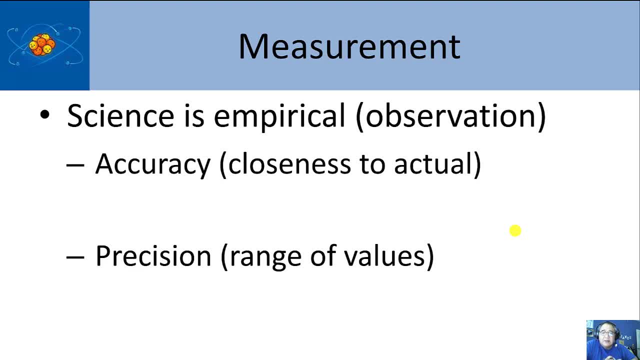 Chemistry, we say, is empirical science. There are also some theoretical sciences that are not based on observation, But an observation would be something like a measurement. okay, So accuracy is really what we refer to when a number is close to what the actual number is. 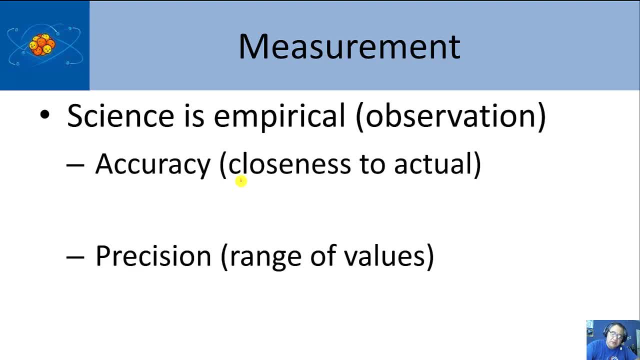 The drawback to accuracy? right, This is closeness to the actual. The drawback to accuracy is that you may not know the actual number, And so you have to make a measurement and hope that it's accurate. But there's also another term, and these two terms get mixed up in our language. 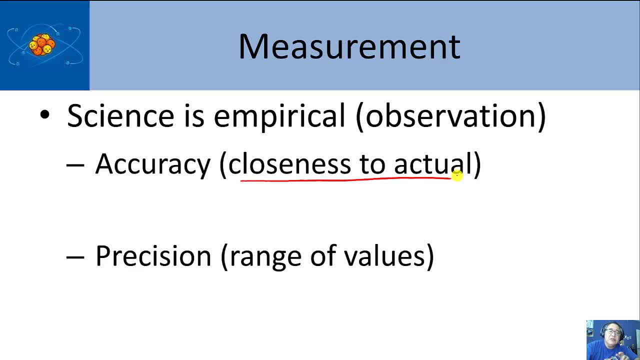 Okay, it's called precision And, in general, what's assumed in science is: if your numbers are precise, then there's a good chance, if you did everything right, that the result is accurate. So what is precision? By the way, that's not necessarily true, okay. 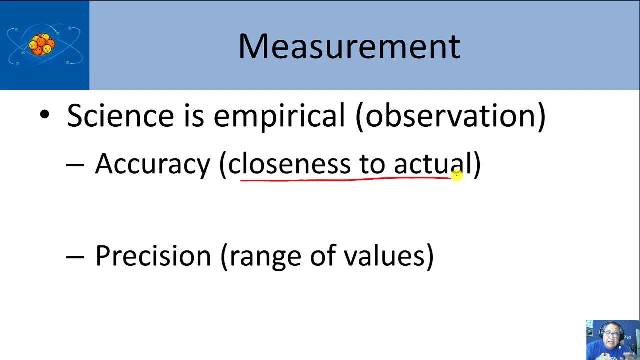 But precision is how close the measured values are to each other. So we refer to that often as the range of the values. And there's a number of ways to characterize the range, And I'm just going to show you a couple in a slide or so. 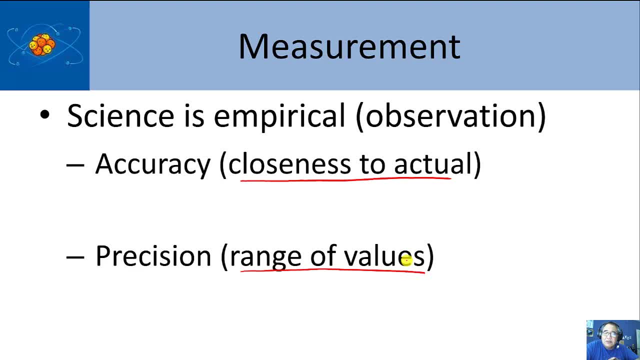 But precision is how close the numbers are to each other. Okay, And so what does closeness mean? In terms of numbers, right, like 3.3 and 3.1, or 3.3 and 3.2, these numbers are closer to each other. 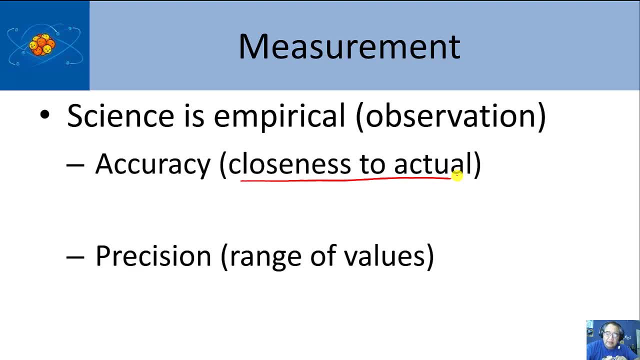 And that's if you did everything right, that the result is accurate. So what is precision? By the way, that's not necessarily true, okay, But precision is how close the measured values are to each other, So we refer to that often as the range of the values. 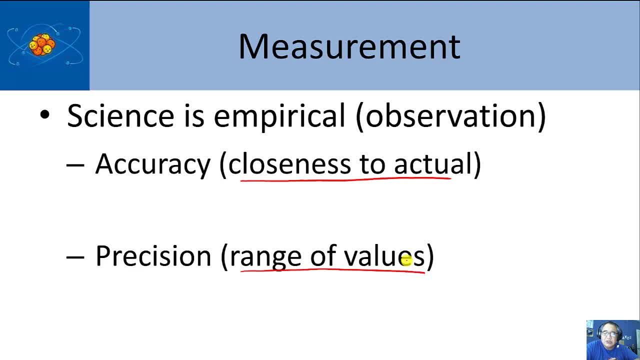 And there's a number of ways to characterize the range, And I'm just going to show you a couple in a slide or so. But precision is how close the numbers are to each other, And so what's assumed in science is that the measured values are close to each other. 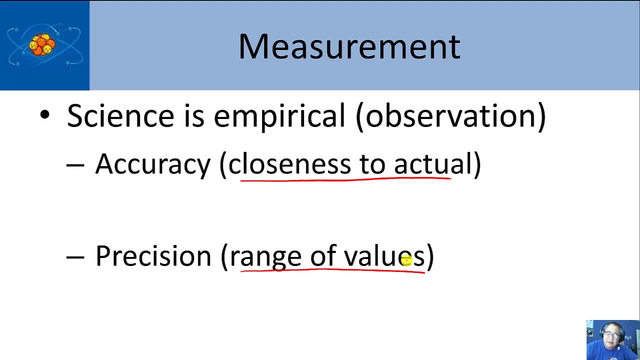 So what does closeness mean? In terms of numbers right like 3.3 and 3.1 or 3.3 and 3.2,, these numbers are closer to each other. That's what we refer to by closeness. 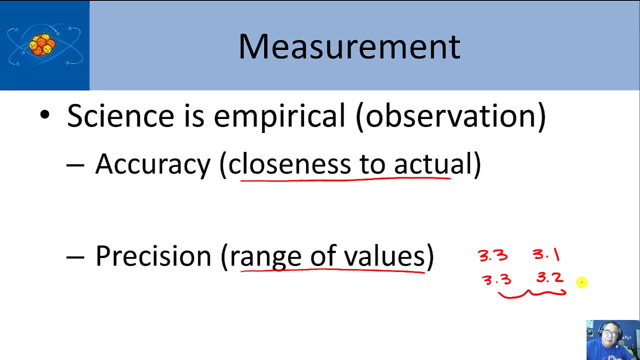 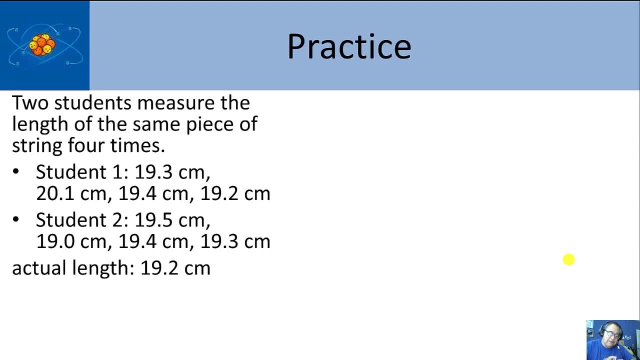 Closer to each other because they're more similar to each other. Now how does that play out in a measurement, right? So let's say you have two students and you give them the same piece of string and they take the same piece of string and they take the same piece of string. 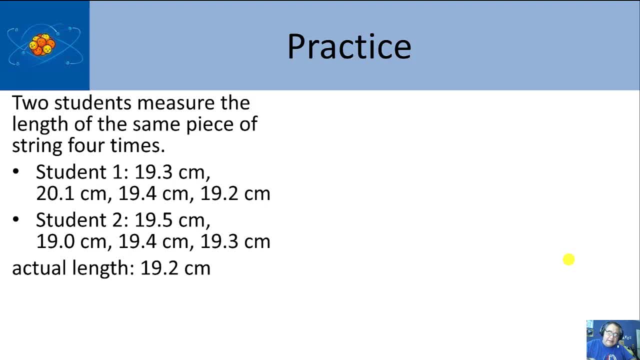 And they measure it four times, right As the teacher in this case. let's say: we know that that's the correct answer, But we're testing their measurement skills. What happens is student one, so we'll call this experiment one. 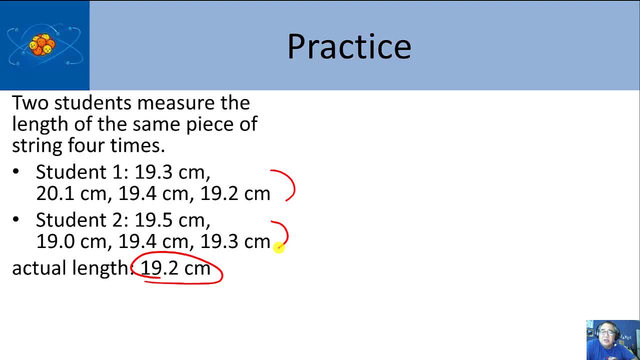 and student two make four measurements, And typically those measurements should not be the same, And usually they're not always exactly the same value, even though you're measuring the same thing. So how do we quantify accuracy and precision? right, So I'm going to show you on the next page. 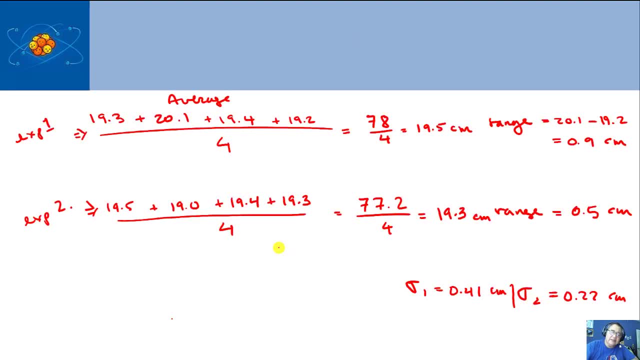 I already wrote a lot of this out. One way to do accuracy is compare it to the average, And so you know when you do an average. I just took the 19.3,, the 20.1,, the 19.4, and 19.2.. 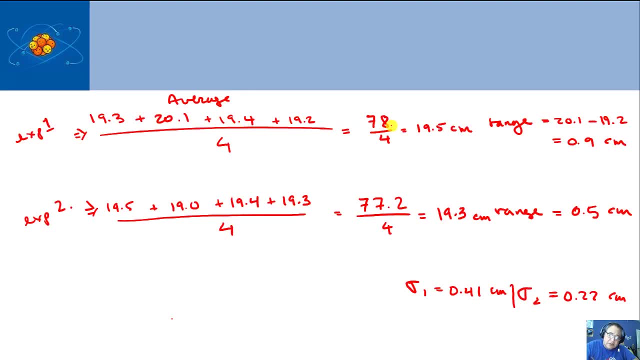 And I added all those together and that actually comes out to 78.0.. Sorry, a little sloppy there. And there are four values. So you take the total right, the sum, and divide it by the number of values you have. 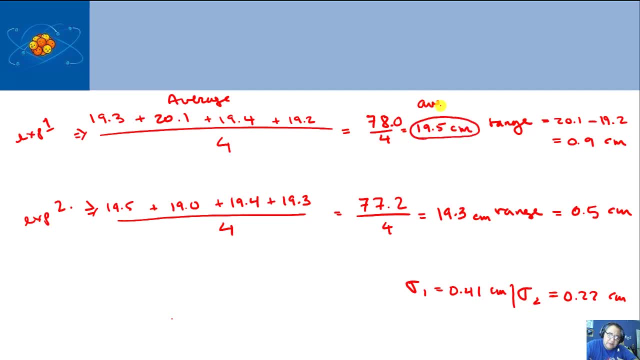 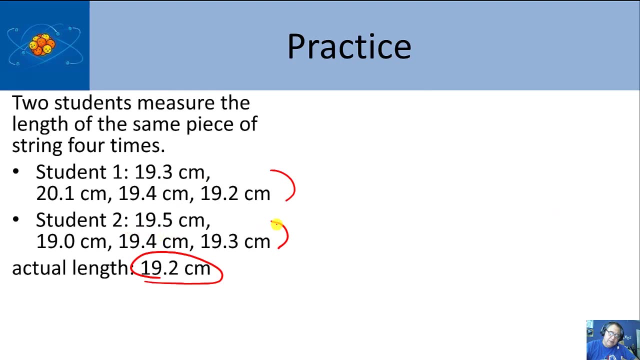 And this is your average right here. So this is my average. And then you can do the same thing with student two's data. Student two has a value of 19.5, et cetera. right, You can see the values there. 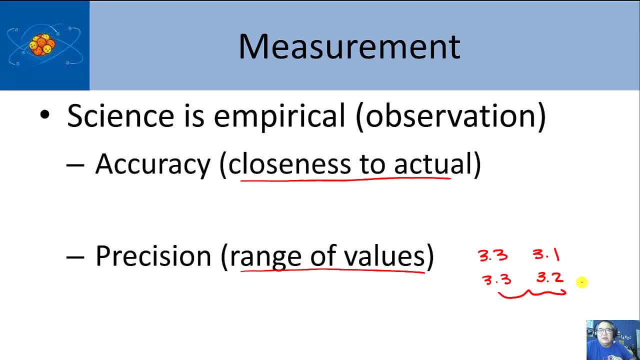 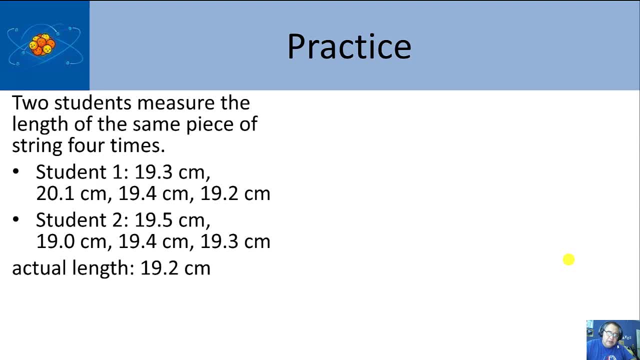 That's what we refer to by closeness: Closer to each other because they're more similar to each other. Now how does that play out in a measurement, right? So let's say you have two students and you give them the same point. 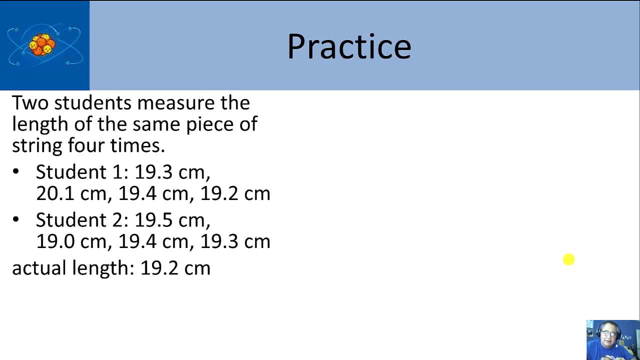 You give them the same piece of string And they take the same piece of string and they measure it four times right As the teacher in this case. let's say we know that that's the correct answer, But we're testing their measurement skills. 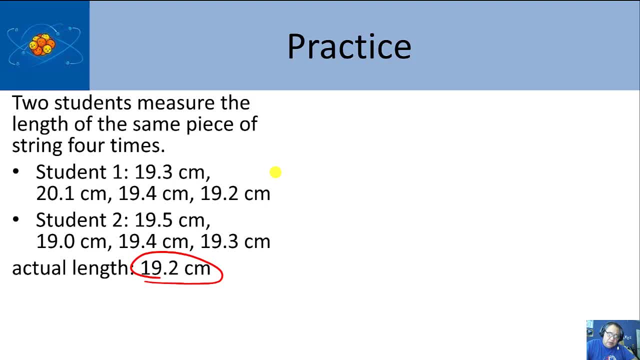 What happens is student one, so we'll call this experiment. one and student two make four measurements, And typically those measurements should not be the same, And usually they're not always exactly the same value, even though you're measuring the same thing. So how do we quantify accuracy and precision, right? 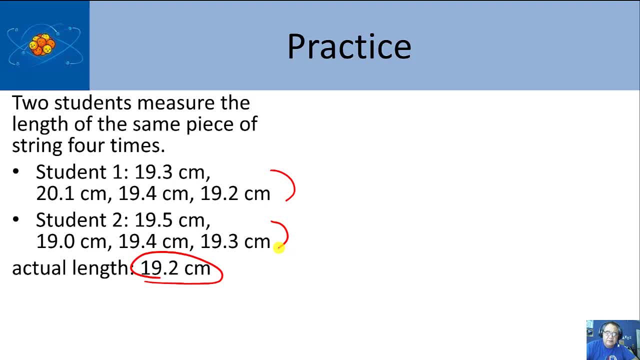 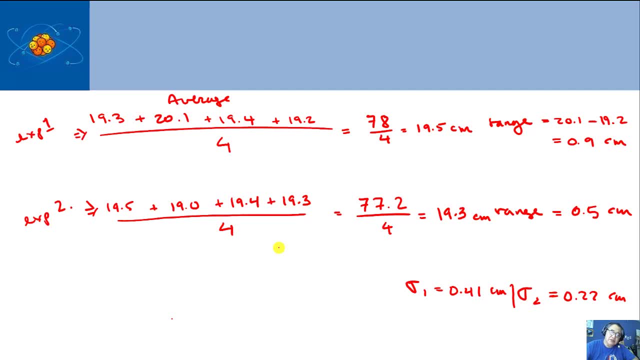 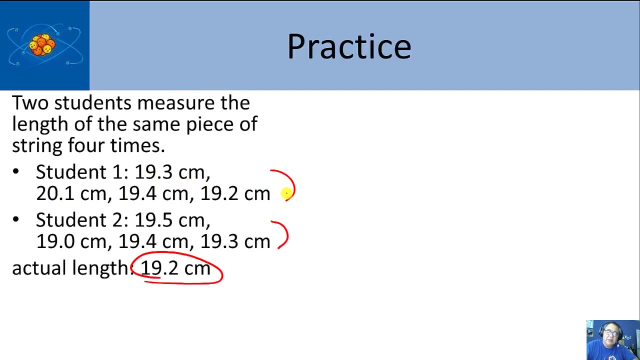 So I'm going to show you on the next page. I already wrote a lot of this out. One way to do accuracy is compare it to the average, And so you know when you do an average. I just took the 19.3,, the 20.1,, the 19.4, and 19.2.. 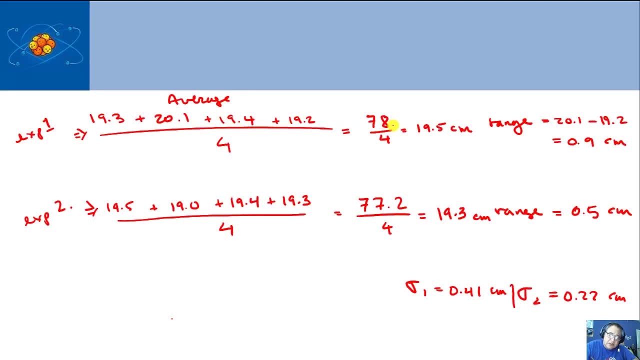 And I added all those together And it actually comes out to 78.0.. Sorry, a little sloppy there. And there are four values. So you take the total right, the sum, and divide it by the number of values you have. 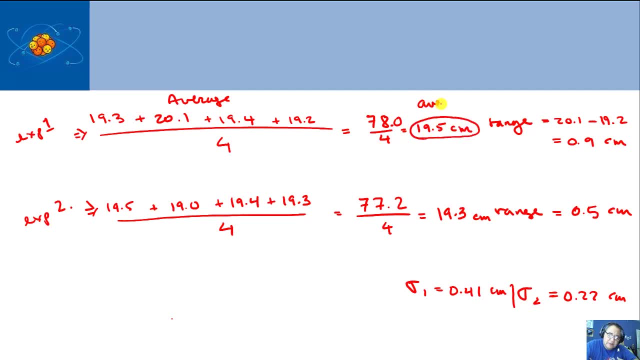 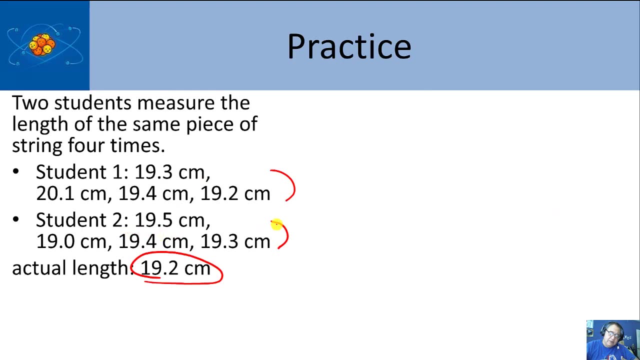 And this is your average right here. So this is my average. And then you can do the same thing with student two's data. Student two has a value of 19.5, et cetera. right, You can see the values there. 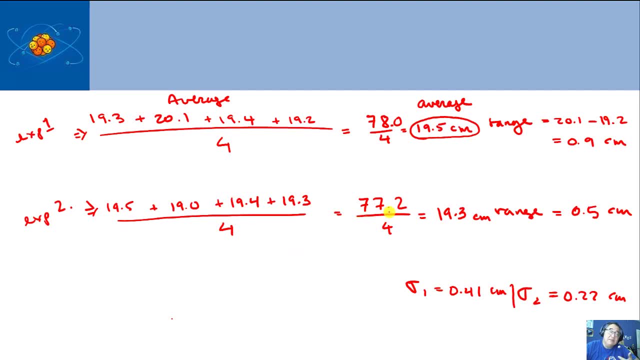 And so I just took all those numbers and I added them together And I got 77.2 as the total or the sum right? This is the sum, that number of those numbers that I'm calculating the average from. Then divide by four and that gives me my average. 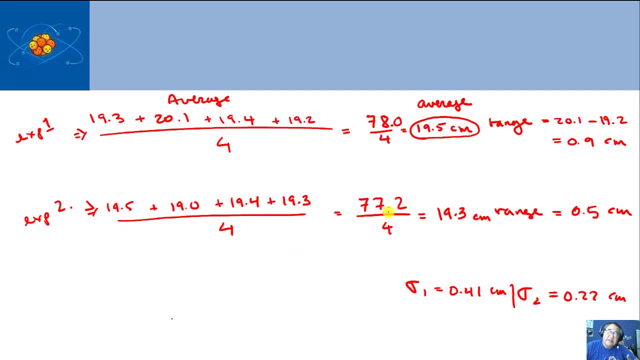 And so I just took all those numbers and I added them together And I got 77.2 as the total or the sum right? So this is the sum, that number of the average, Those numbers that I'm calculating the average from. 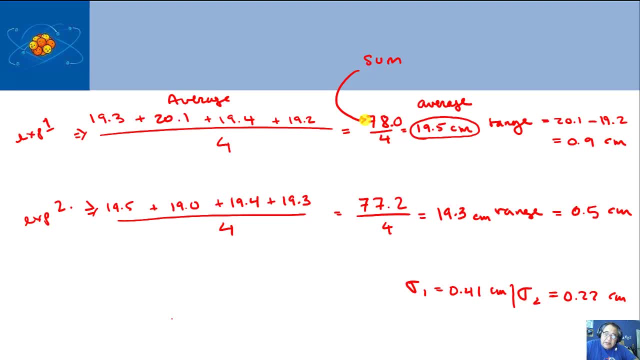 Then divide by four and that gives me my average. So I ended up with 19.3.. Now, as the teacher in this instance, right, we know, the answer is 19.2.. So actual is 19.2.. 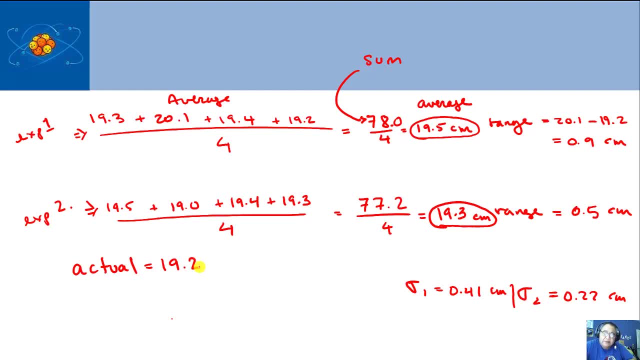 Now, whose number is more accurate, right? Well, if you look at the student results, you'll notice that 19.3 is closer than 19.2, than 19.5 is, So we can already say that this one is more accurate. 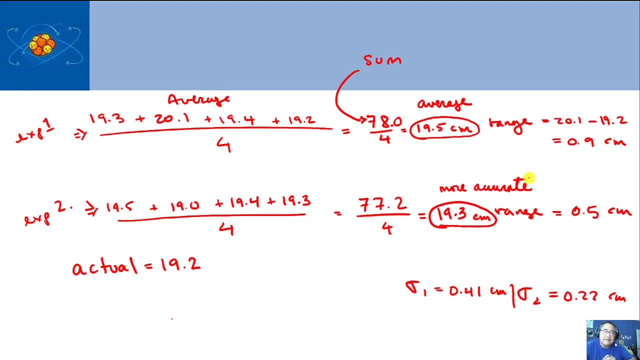 Now we can quantify that as a percent, right, as a percent of the actual, And the way that that's done is this is going to be called the percent error, So it makes it set And then, like you know, it's not going to be礼 0.. 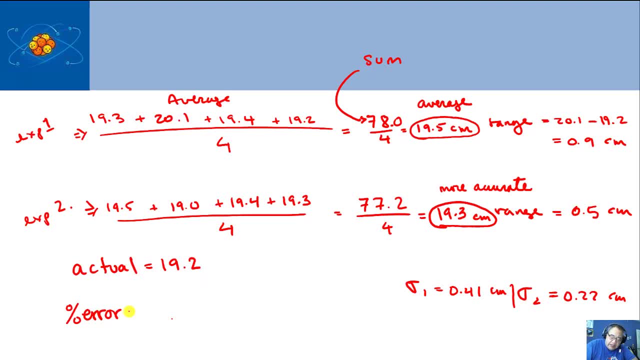 It looks like a pretty good average right, But we're going to calculate how much error there is in that measurement And then the way we do that actually is the measured minus the true value divided by the true value times. or, if you're in the real world, it's going to be like: 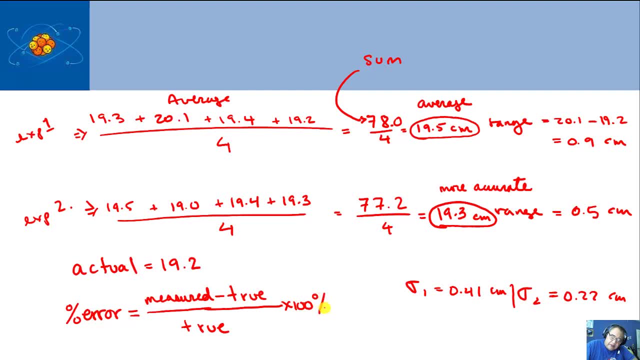 and then I'm going to measure it right: 100%. so this is the true value, the actual value. so let's go ahead and do that calculation. I'm gonna whip out my handy-dandy calculator over here, this one which I actually like. I keep telling you guys I don't really like it, but I 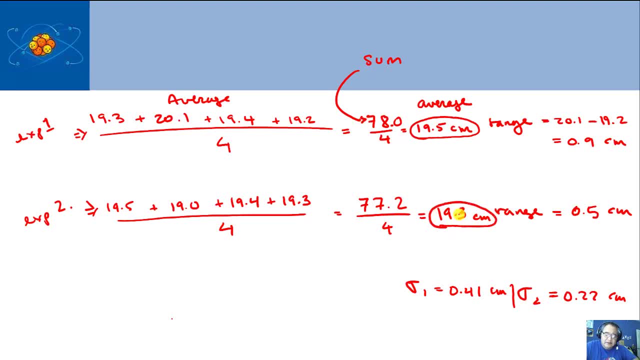 So I ended up with 19.3.. Now, as the teacher in this instance, right, we know, the answer is 19.2.. So actual is 19.2.. Now, whose number is more accurate, Right? Well, if you look at the student results, you'll notice that 19.3 is closer to 19.2 than 19.5 is. 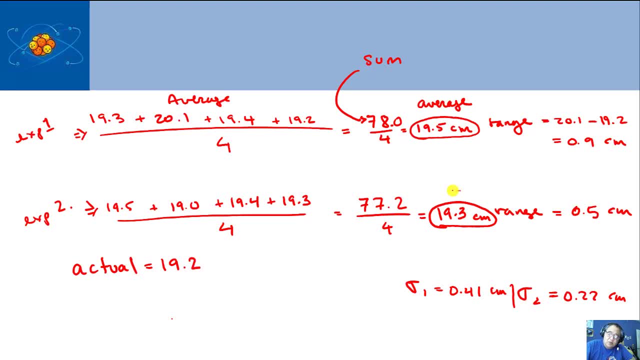 So we can already say that this one is more accurate. Now we can quantify that as a percent right, as a percent of the actual, And the way that that's done is this is going to be called the percent error, So it makes it sound bad. 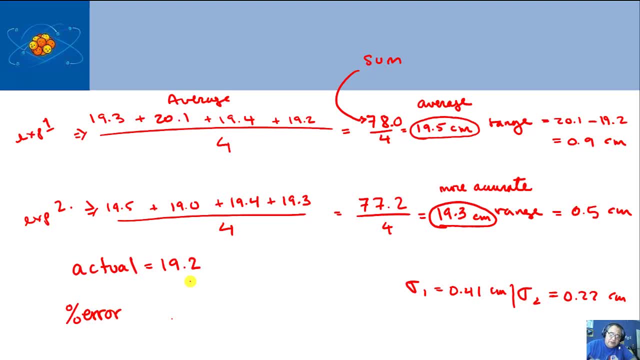 Like we know, it looks like a pretty good average, right, But we're going to calculate how much error there is in that measurement And then the way we do that actually is the measured minus the true value Minus the true value divided by the true value times 100%. 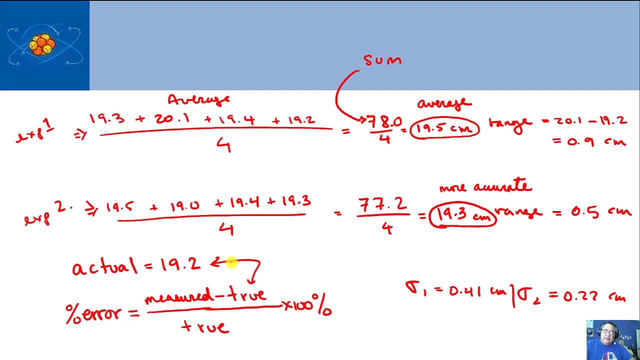 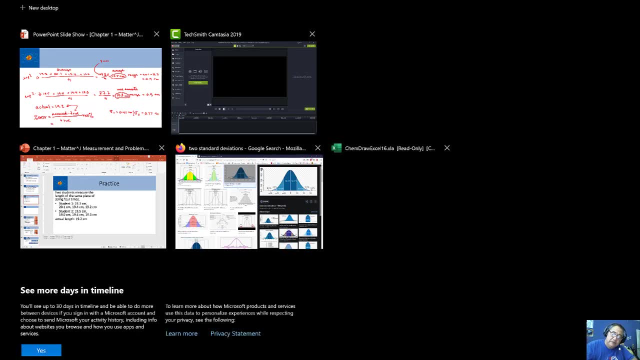 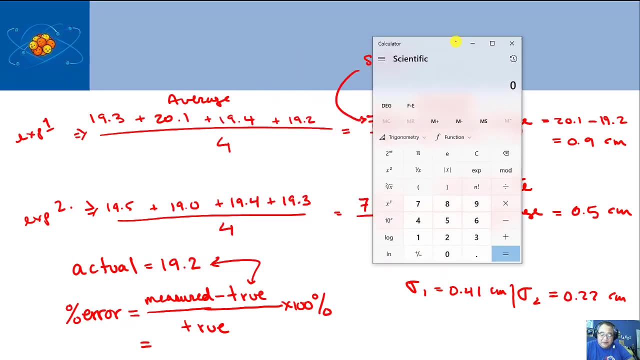 So this is the true value, the actual value. So let's go ahead and do that calculation. I'm going to whip out my handy dandy calculator over here, This one which I actually like. I keep telling you guys I don't really like it, but I don't know if a better one for the computer. 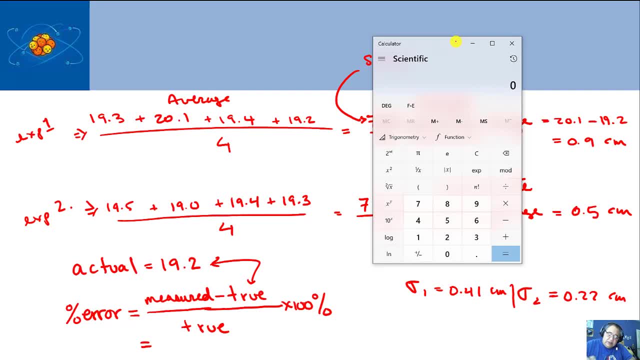 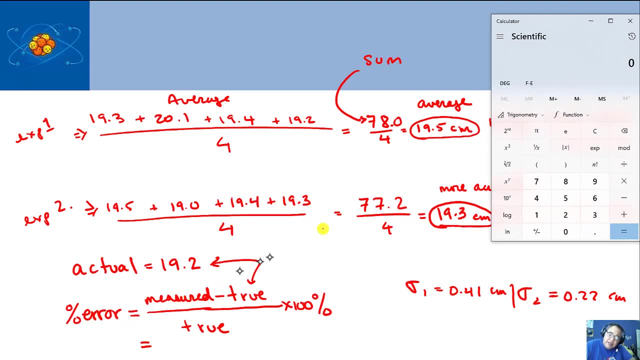 that you can actually see me do the calculations on. So that's going to be oops. sorry, I didn't write it out. That's going to be the measured value, the average 19.5 minus 19.2.. 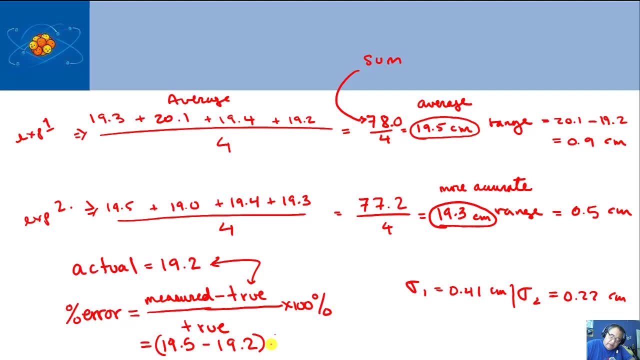 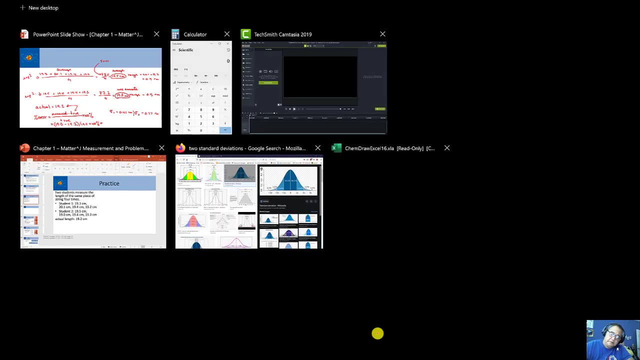 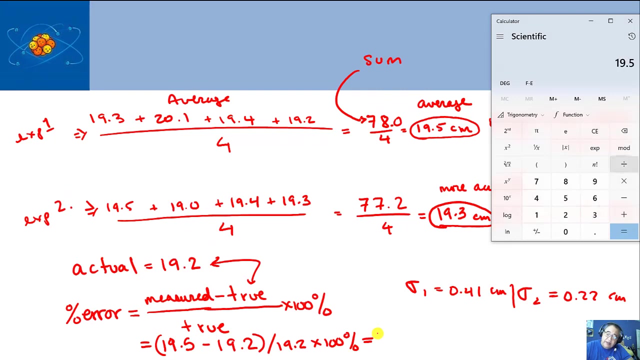 So this is for experiment, one Divided by 19.2 times 100%. So let's pull up the calculator again. So 19.5 minus 19.2.. I'll hit equals, and then I'll go divided by 19.2.. 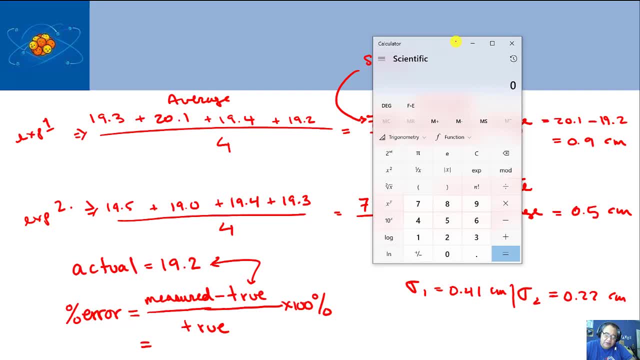 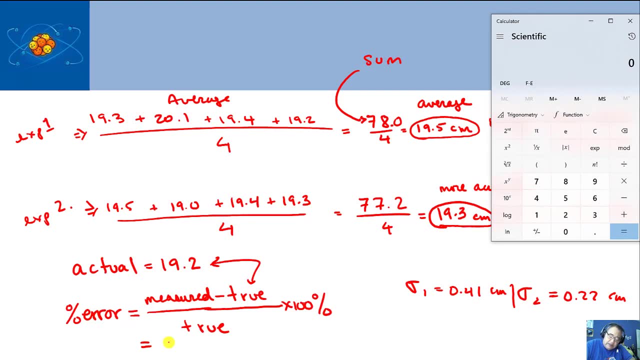 don't know if a better one for the computer that you can actually see me do the calculations on. so that's gonna be sorry, I didn't write it out. that's gonna be the measured value, the average nineteen point five minus nineteen point two. so this is for experiment, one divided by nineteen point two times one. 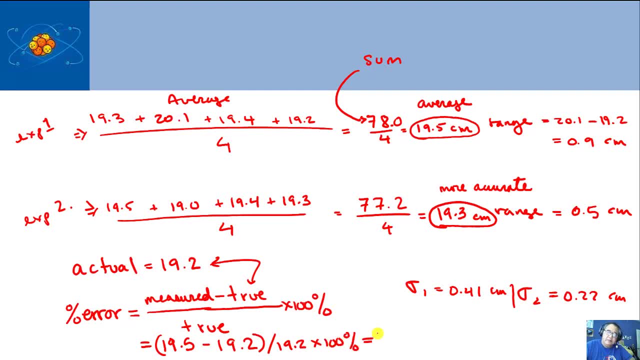 hundred percent. so let's pull up the calculator again. so 19.5 minus 19.2, I'll hit equals. and then I'll go divided by nineteen point two times 100 to get my percent, and that becomes point. we'll call it one point six percent. 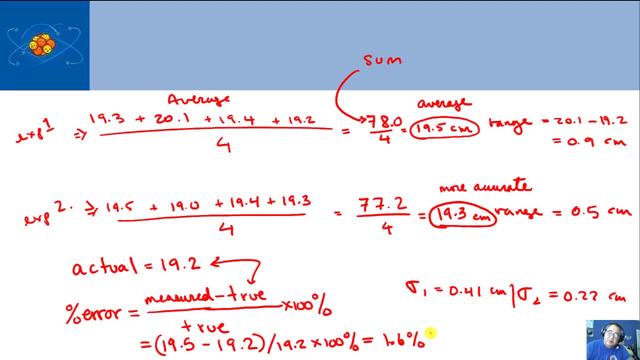 okay, so let's look at the other one. I didn't really leave myself enough space here, did I? but let's go ahead and try to do that. we'll do the other one at the top. so the percent error for this is for trial, trial one or experiment one for. 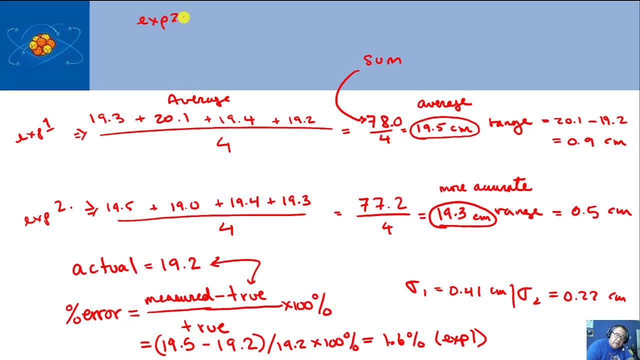 experiment two. we can do the same thing I can do. let's see what is it. it's nineteen point three. so this is the measured value. all right, minus nineteen point two, divided by nineteen point two. again, again, you divide by the known value times one hundred percent. 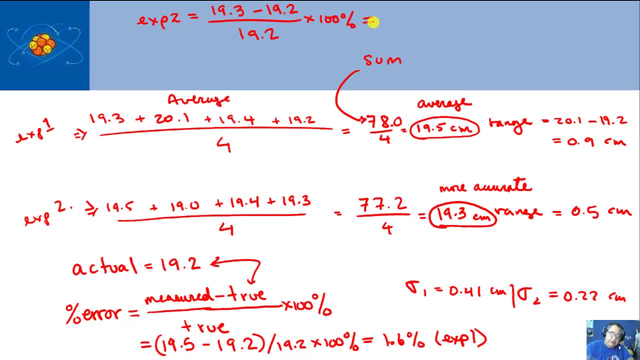 and that's it for the experiment two. we can do the same thing I can do. let's see what's going on here. we can do the same thing. we can do the same thing we can do. that will come out to be we'll pull up the calculator real quick. I'm not sure. 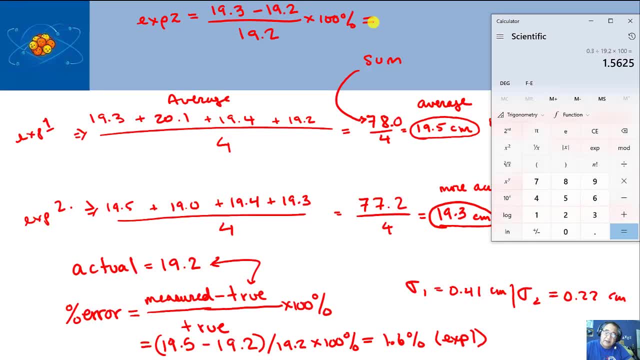 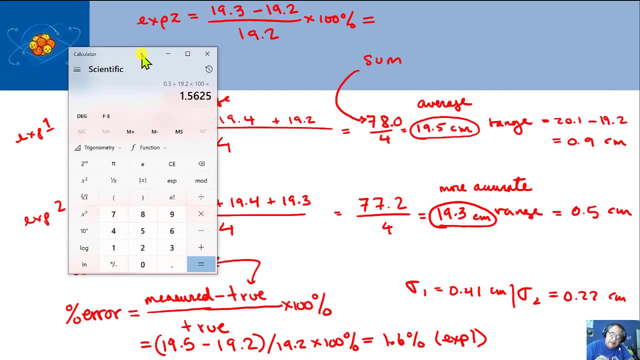 what my computer is doing, but it's like on overdrive and getting super hot, so I may have to stop here for a little bit. hopefully I don't get too disconnected. so let's see, here we go. yeah, nineteen point three minus nineteen point two, which I 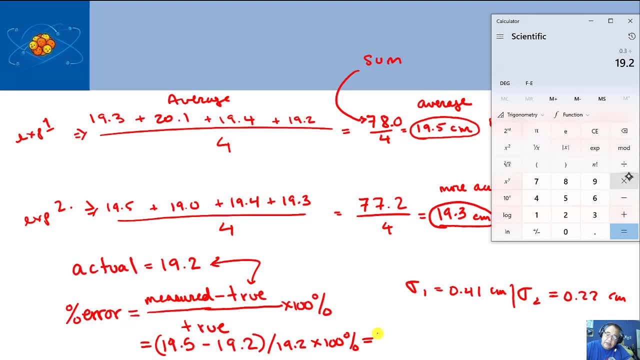 Times 100 to get my percent, And that becomes 1 point. we'll call it 1.6%. Okay, so let's look at the other one. I didn't really leave myself enough space here, did I? But let's go ahead and try to do that. 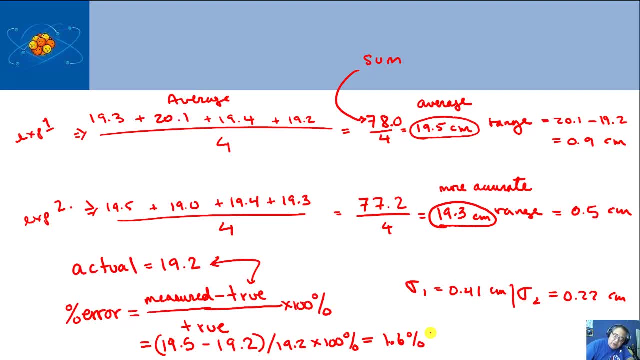 We'll do the other one at the top. So the percent error: this is for trial one or experiment one. For experiment two, we can do the same thing I can do. let's see what is it. It's 19.3,. so this is the measured value. 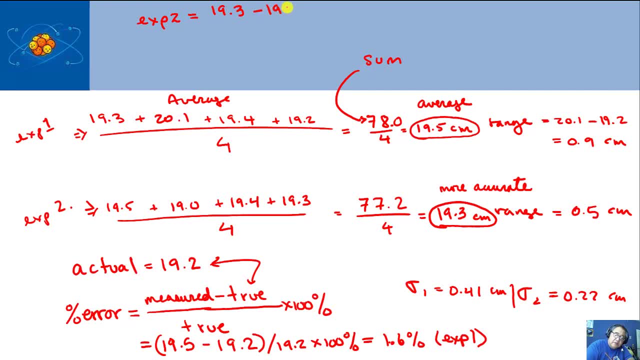 minus 19.2.. Divided by 19.2, again Again, you divide by the known value times 100%, And that will come out to be: we'll pull up the calculator real quick. I'm not sure what my computer is doing. 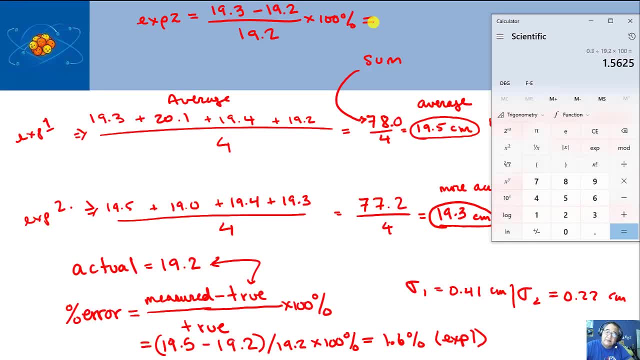 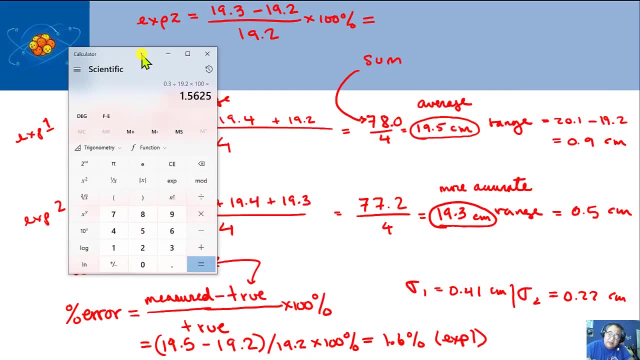 but it's like on overdrive and getting super hot, so I may have to stop here for a little bit. Hopefully I don't get too disconnected. So let's see, here we go. Yeah, 19.3 minus 19.2,. 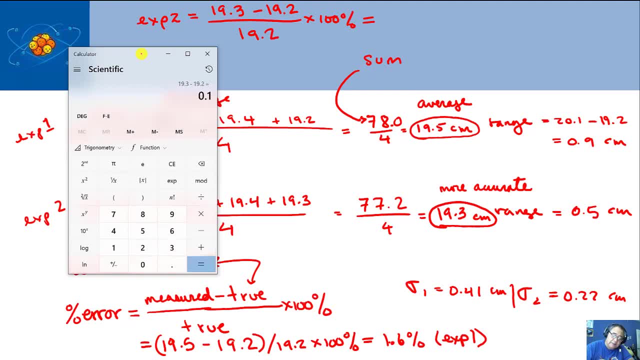 which I should have probably just written: .1, divided by 19.2.. And then times 100,, 0.52%. Okay, So when you're looking at the error in those values- like the accuracy error, right- Then what we find is again: this value is smaller, right. 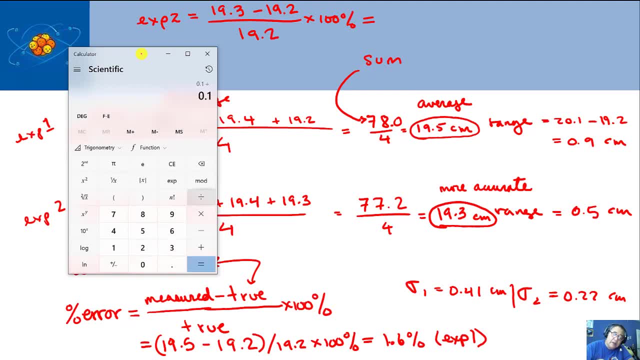 should have probably just reduced it to one point six percent. so that's the just written point one divided by nineteen point two and then times a hundred zero point five, two percent. so when you're looking at the error in those values like the, the accuracy error right. 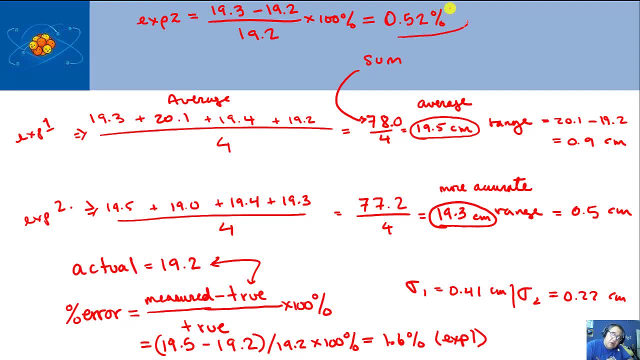 then what we find is again this value smaller, right, because the value that was measured is actually closer to the known or accepted value or the true value, okay, okay. so that's, that's one aspect: the accuracy, how close it is to the actual value. the other value, other idea, is called the precision, and we'll do that. 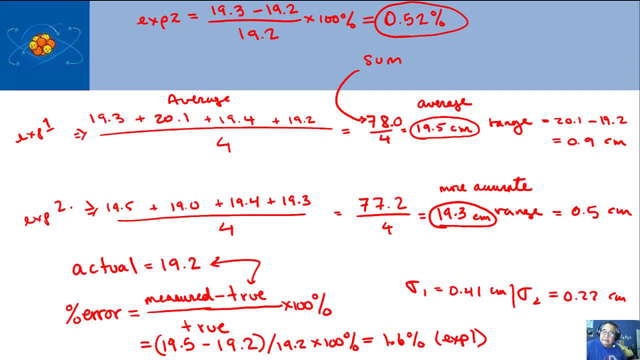 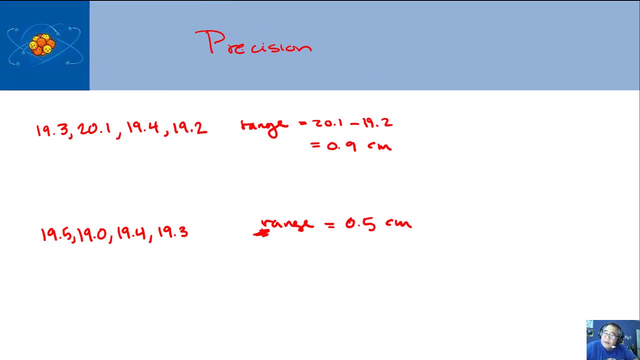 on the next slide. so another aspect that we deal with is known as precision, and so I've just recopied the numbers here from the original data. so this is experiment one or student one, and this is experiment two. right, and what we find is that that 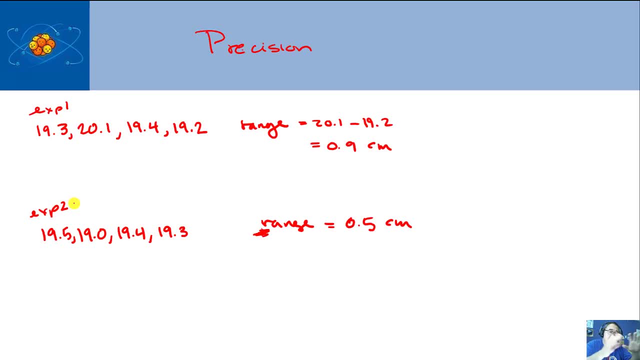 if you want to know what the precision is is that you need to see how close the numbers are together. and in measuring the close of the numbers that gives you an idea how precise they are is how, how repeatable they are. so precision is really telling us. how well could you? 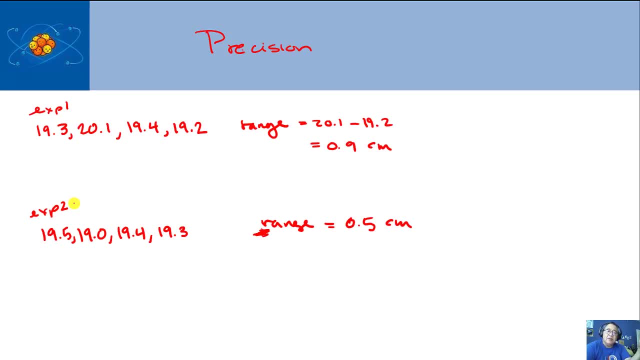 repeat this measurement. get a similar number if you did it again. okay. so in this case, the simplest way, and probably the first way people learn to deal with this, is called looking at the range of the numbers, and the range is really what it sounds like. you take the high number and the low number, so in this case, I'm 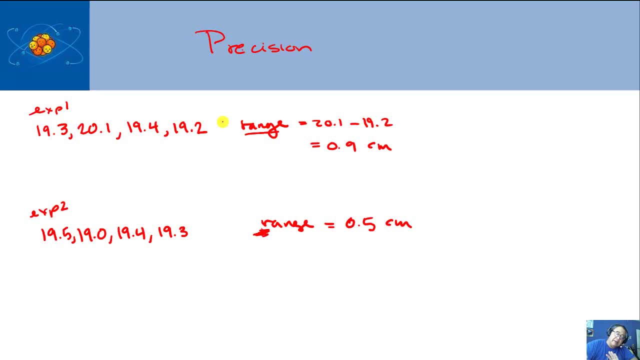 looking through the list now. oftentimes people will sort the list from low to high- okay, or high to low, either way- and then look to see which one is the first number and the last number. so if I were to do that, right, nineteen point two is the lowest number and twenty point one. 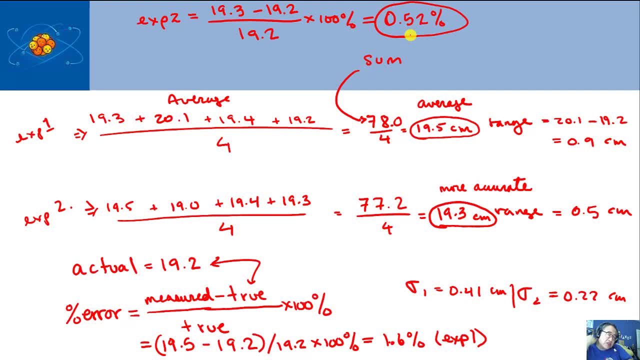 Because the value that was measured is actually closer to the known or accepted value, or the true value, okay, Okay. so that's one aspect: The accuracy, how close it is to the actual value. The other idea is called the precision. 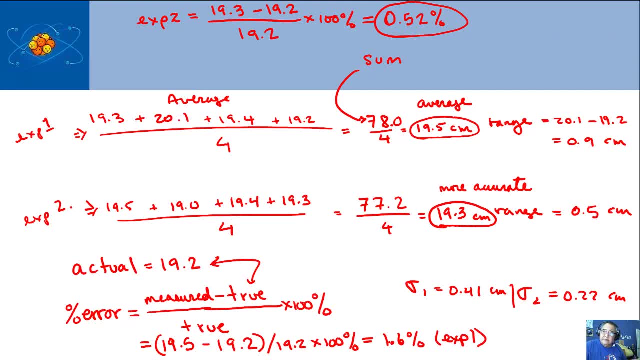 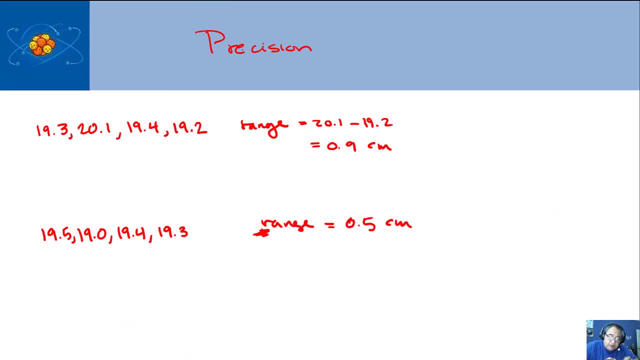 and we'll do that on the next slide. So another aspect that we deal with is known as precision, And so I've just recopied the numbers here from the original data. So this is experiment one, or student one, And this is experiment two, right, 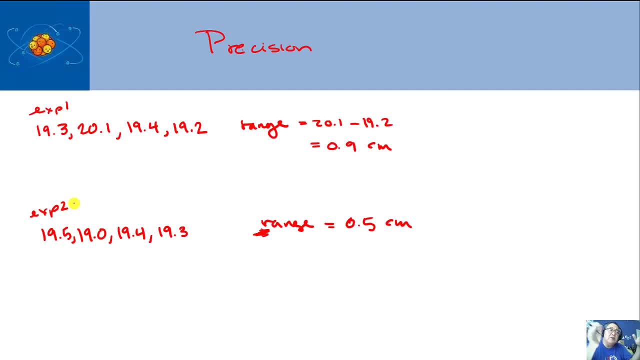 And what we find is that if you want to know what the precision is, is that you need to see how close the numbers are together. And in measuring the closeness of the numbers, that gives you an idea how precise they are, how repeatable they are. 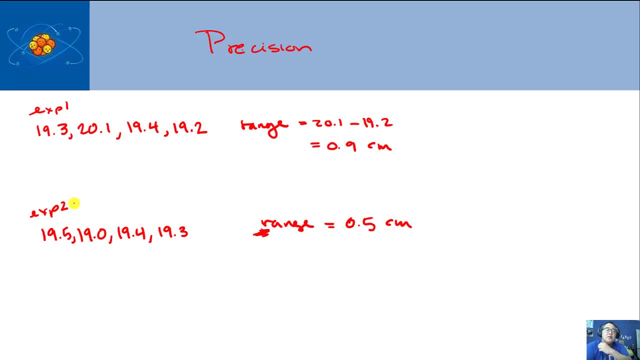 So precision is really telling us. how well could you repeat this measurement, get a similar number, if you did it again? Okay, so in this case, the simplest way, and probably the first way people learn to deal with this, is called looking at the range of the numbers. 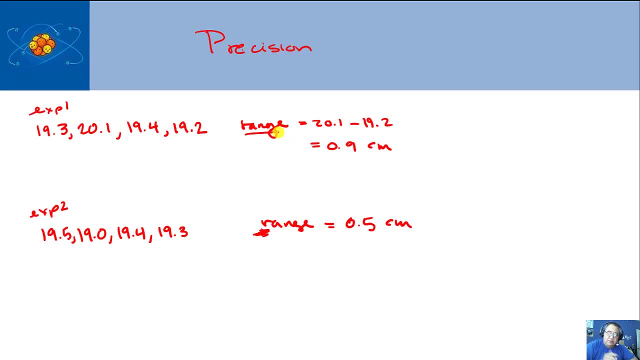 And the range is really what it sounds like. You take the high number and the low number, So in this case, I'm looking through the list Now. oftentimes people will sort the list from low to high. okay, Or high to low, either way. 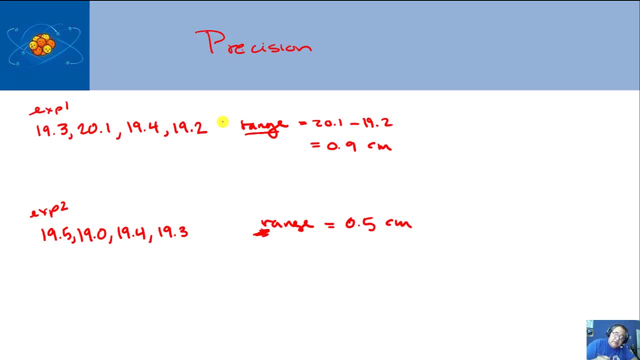 And then look to see which one is the first number and the last number. So if I were to do that right, 19.2 is the lowest number and 20.1 is the highest number, and those would be on opposite ends. 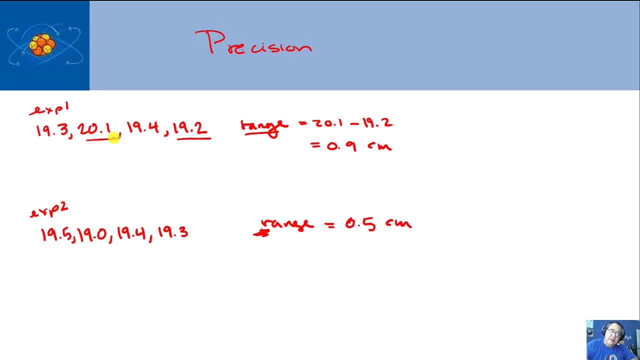 And the range is usually calculated as an absolute value, And so, in this case, 20.1 minus 19.2 gives me a range of 0.9 centimeters. Now, if I did that with Experiment 2, what would happen is I would look at these numbers. 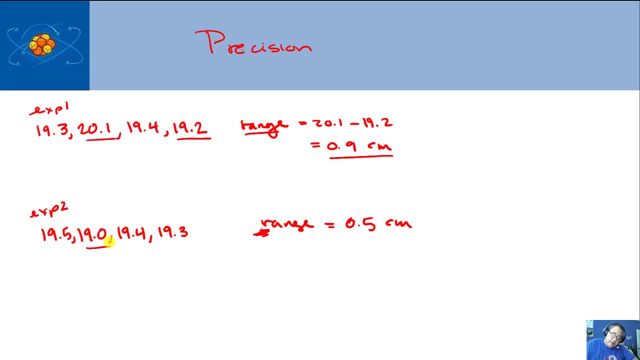 and I would look for the lowest and it looks like this is my lowest, And then, if I look for the highest, it looks like this is my highest one, And so 19.5 minus 19.0, that gives me a range of 0.5. 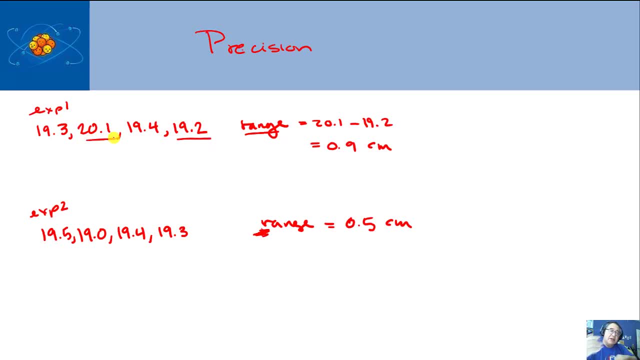 is the highest number, and those would be on opposite ends, and the range is usually calculated as an absolute value. and so, in this case, night twenty point one minus nineteen point two gives me a range of point nine centimeters. now, if I did that with experiment two, what would happen? 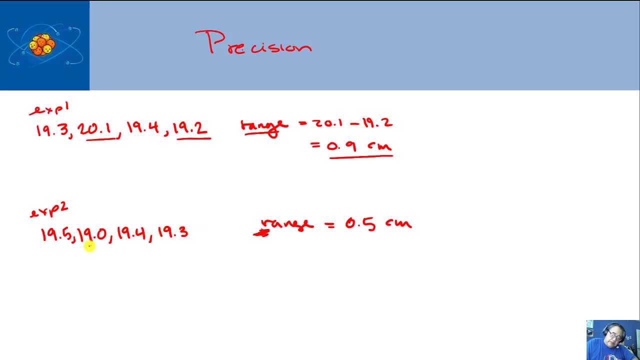 is is. I would look at these numbers and I would look for the lowest and it looks like this is my lowest, and then, if I look for the highest, it looks like this is my highest one. and so nineteen point five minus nineteen point zero, that gives me a range of point five. now I'm not going to cover, so, anyways, which one of 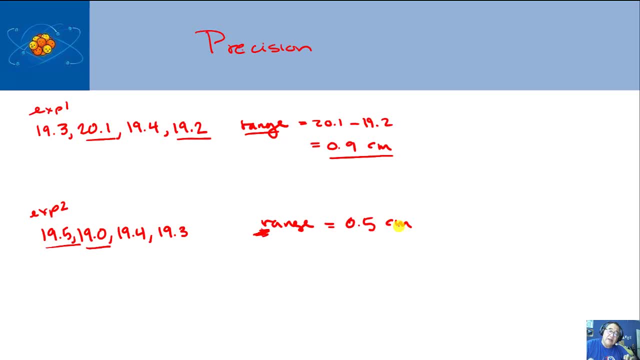 these two sets is more precise, right? the more precise value set of numbers is actually experiment two, even though experiment one appears to be more accurate. okay, so those are. that's the difference. experiment two: it looks like if that person made the measurement again, they would get a. 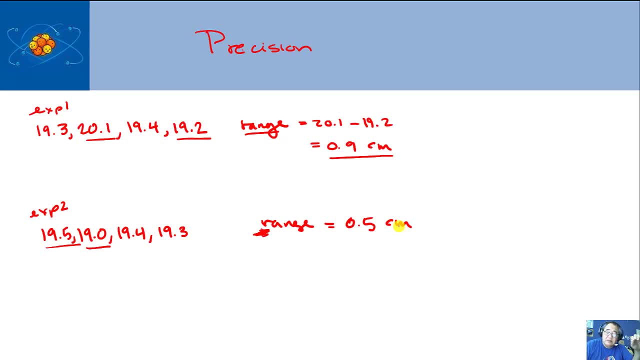 result that is similar to the original measurements right. on the other hand, accuracy is how closely when you do your measurements are you getting to the actual number? and really that's the gold standard. that's what we want to do, but oftentimes we don't know what the actual number is. the first time, like I was. 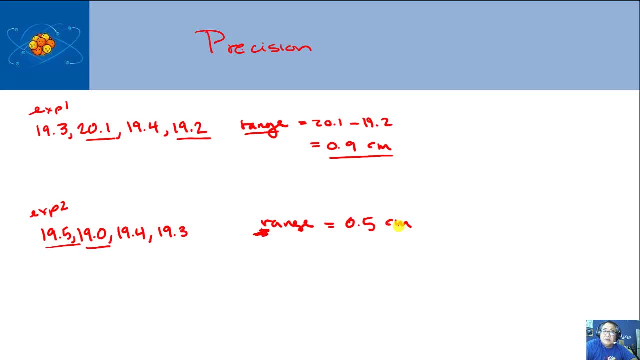 talking about earlier, we we determine the number of molecules inside a vesicle. that's what we did. we were able to count them. basically, then, what happened was we made lots and lots of measurements, and so we had an idea about the range of the sizes, but we really 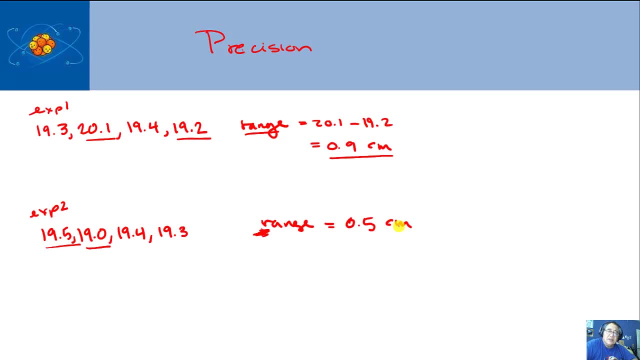 didn't know how accurate that number was, and so we had to do actually a large literature search. actually my friend did it, largely because it was his project. he did the large literature search and try to figure out: well, what do we actually know about, how much is each and each vesicle? and so that's where we were able. 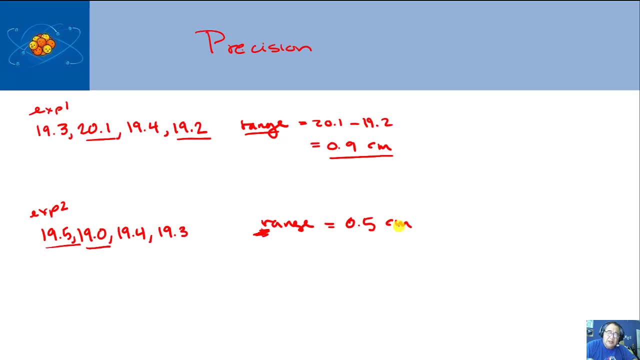 to look at our data and say it's consistent with the other day and then sort of point out why you know the way we were doing is maybe better or worse, for that matter. okay, now I'm going to talk about it here. this is actually a lab topic, but there's also something called the standard deviation and this: 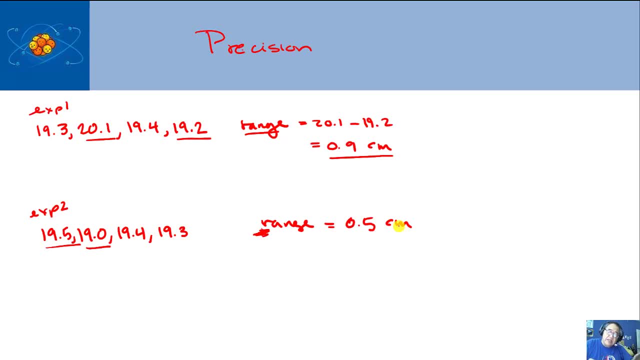 Now I'm not going to cover. So anyways, which one of these two sets is more precise, right? The more precise value set of numbers is actually Experiment 2, even though Experiment 1 appears to be more accurate. Okay, so that's the difference. 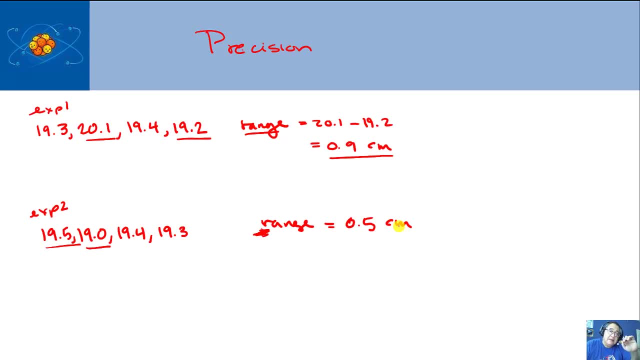 Experiment 2,. it looks like if that person made the measurement again, they would get a result that is similar to the original measurements, right? On the other hand, accuracy is how closely when you do your measurements, are you getting to the actual number? 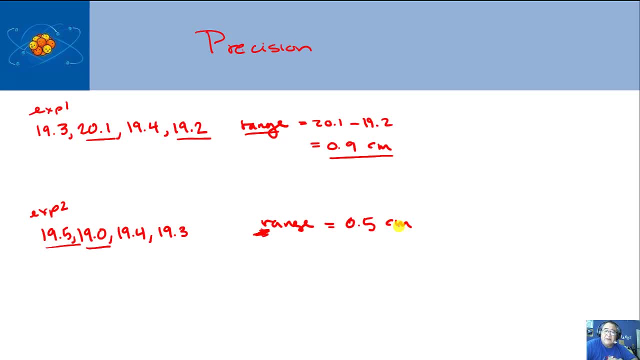 And really that's the gold standard. That's what we want to do, But oftentimes we don't know what the actual number is. The first time, like I was talking about earlier, we determined the number of molecules inside a vesicle. 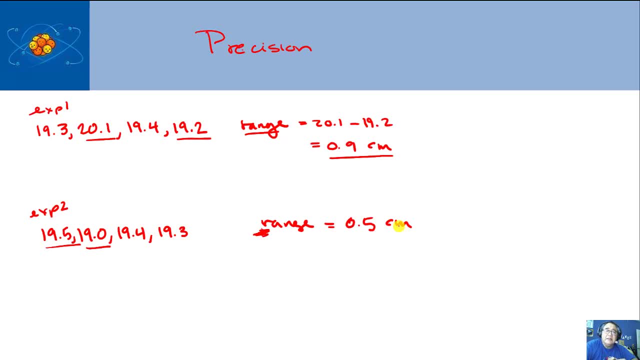 That's what we did. We were able to count them basically. Then what happened was we made lots and lots of measurements And so we had an idea of- We were thinking about- the range of the sizes, but we really didn't know how accurate that number was. 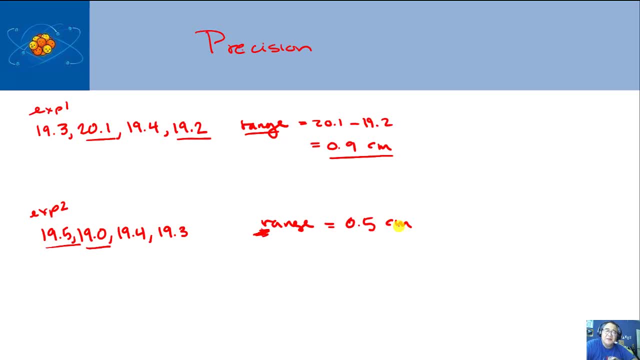 And so we had to do actually a large literature search. Actually my friend did it because it was his project. He did the large literature search and tried to figure out: well, what do we actually know about? how much is each in each vesicle? 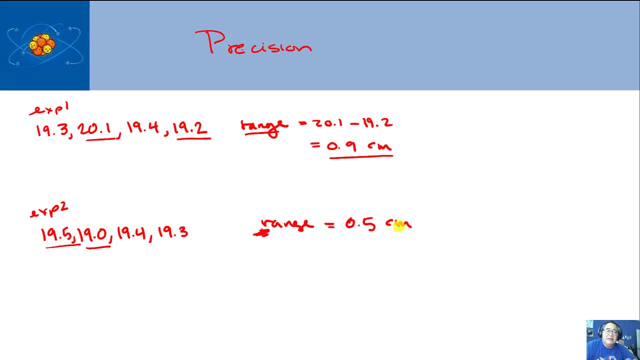 And so that's where we were able to look at our data and say it's consistent with the other data and then sort of point out why the way we were doing it is maybe better or worse, for that matter. Okay, now I'm not going to talk about it here. 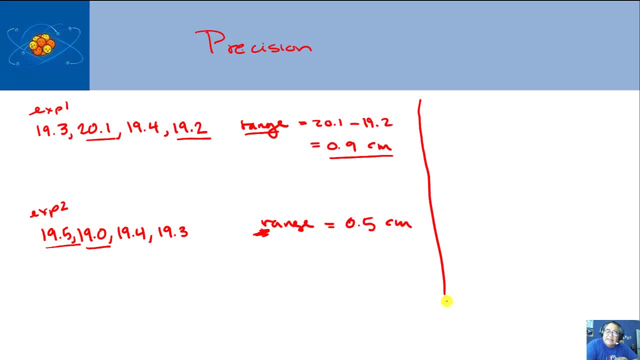 This is actually a lab topic, But there's also something called the standard deviation, And this is what most scientists use for sets of data like this, And if you look at the top set of numbers, what we get is a standard deviation. It's experiment one. 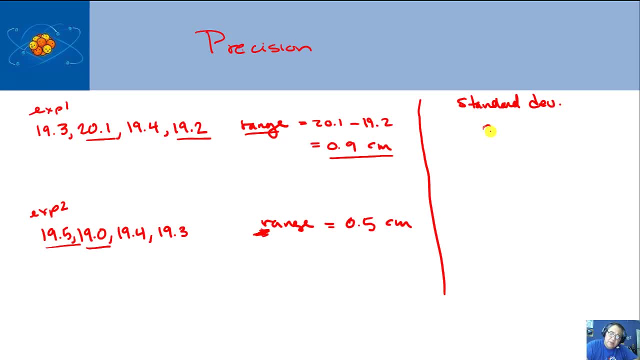 We get a standard deviation of 0.41.. And the symbol that's usually given to it is S Or S right like that. And then for the second set of numbers, the standards for experiment two, the standard deviation or sigma. 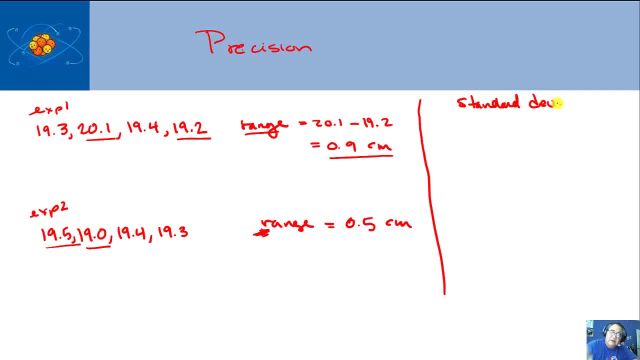 is what most scientists use for sets of data like this, and if you look at the top, top, top- a set of numbers- okay, what we get is a standard deviation. it's experiment one. we get a standard deviation of 0.41, and the symbol that's usually given to it is: 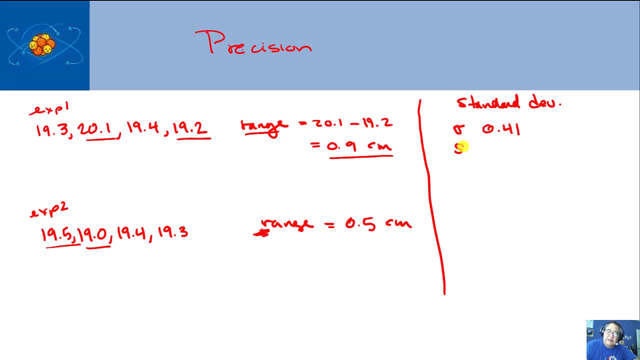 s or s right like that. and then for the second set of numbers, the standards for experiment to the standard deviation, or Sigma, is 0.22. okay, again, it agrees with the range and you and, in that the standard deviation for the second set of numbers is smaller than the set of standard deviation for the first set of numbers. 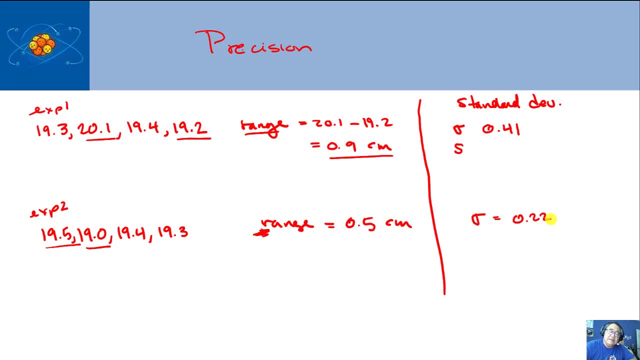 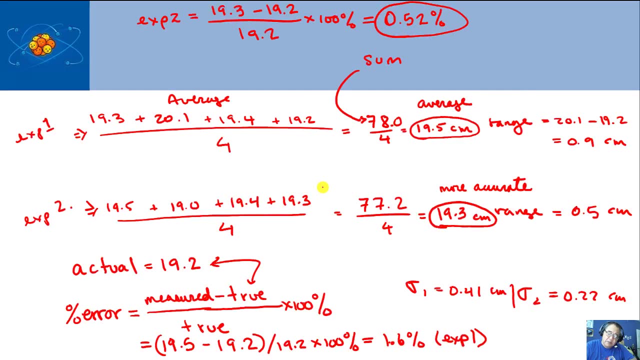 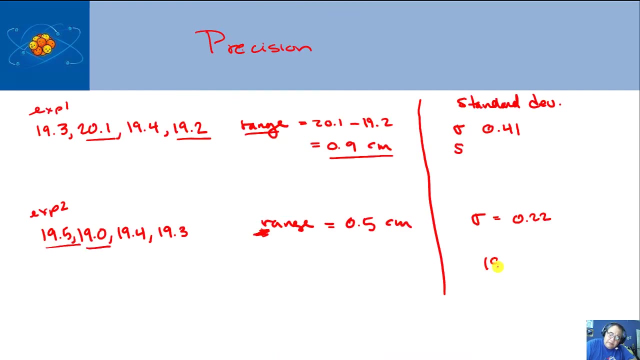 the interesting thing about the standard deviation is statistically what it means. okay, so I got my. I've got my average. to go back for a second, for let's look at experiment twos average. the average was 19.3 right, so the average is 19.3 if I. 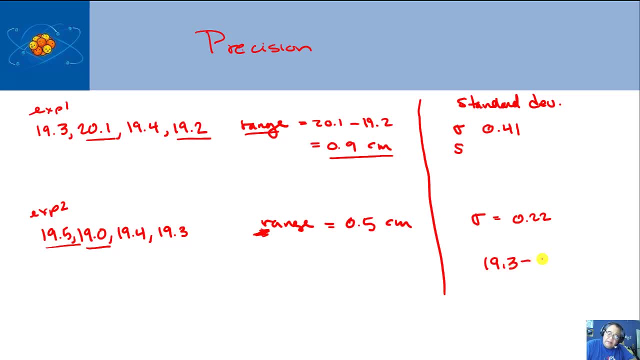 subtract 0.22 from that, I'm going to get, let's see 19.11. and if I add it to their 19.3 plus 0- sorry 0.22- then I'll end up with 19.52 like that. so in terms of like number lines, 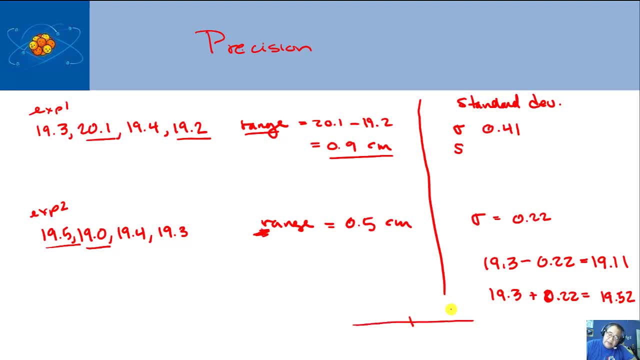 right. so I had a number line and this is 19.3, and then I have these two values. I just calculated I had 19.11 and 19.52. alright, what? what the standard deviation is telling me mathematically what it does is: 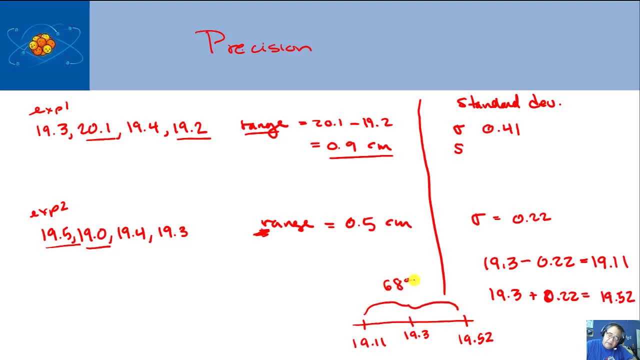 it turns out about 68% of the values that you measure based on that standard deviation should fall within that. no, it will say 0.225. so in the case of that, we got 3.60 of 5 aight. so if I have 279.82, 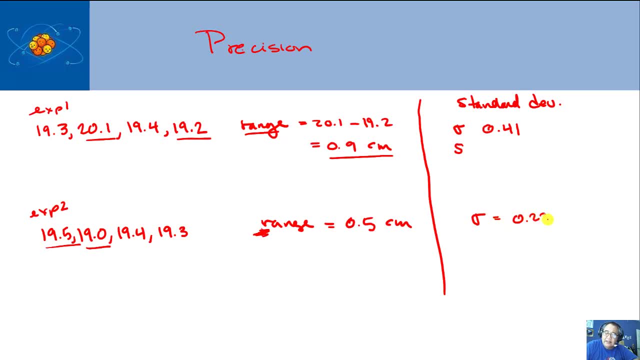 is 0.22.. Again, it agrees with the range, And the standard deviation for the second set of numbers is smaller than the set of standard deviation for the first set of numbers. The interesting thing about the standard deviation is, statistically, what it means. 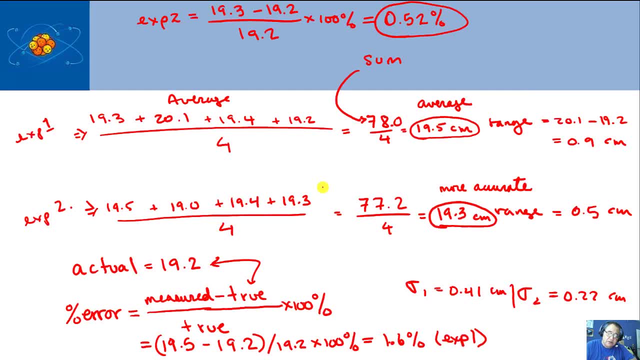 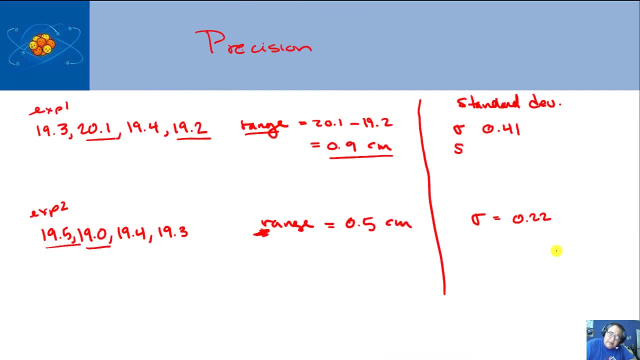 Okay, so I've got my average. Let's go back for a second. Let's look at experiment two's average. The average was 19.3, right? So the average is 19.3.. If I subtract 0.22 from that, 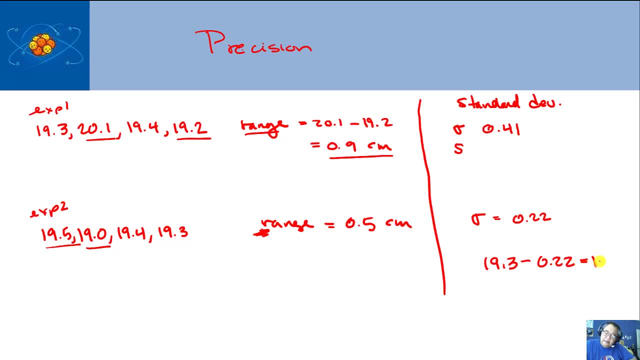 I'm going to get, let's see, 19.11.. And if I add it to there, 19.3 plus 0.22, then I'll end up with 19.52,, like that. So in terms of like number lines, right. 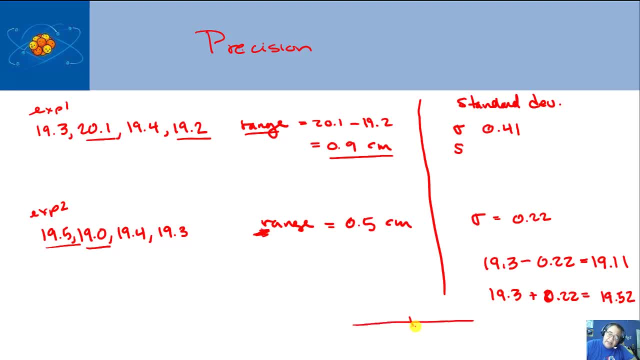 so if I had a number line, and this is 19.3, and then I have these two values, I just calculated I had 19.11, and I had 19.52,. right What the standard deviation is telling me. 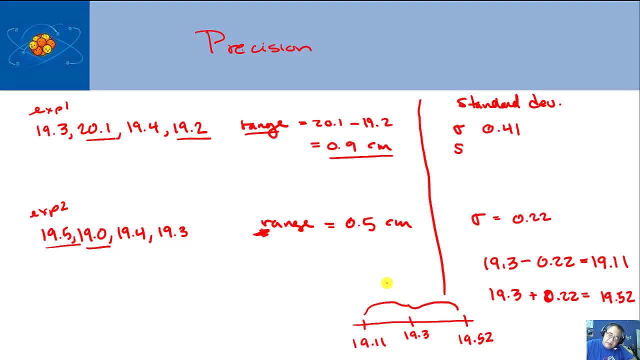 mathematically what it does is. it turns out about 68% of the values that you measure based on that standard deviation should fall within that range. If you do two standard deviations, it turns out 95% of the values you measure using the same technique should fall in that range. 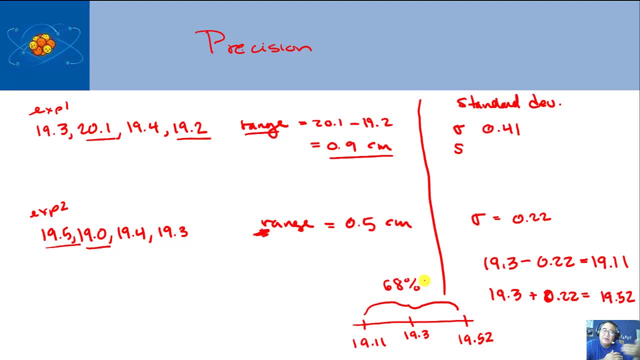 So then the thing is is if a number falls outside of that range, we have a good guess that it belongs to a different set of data, For example the set of data that has errors in it, or maybe from a different population of measurements. 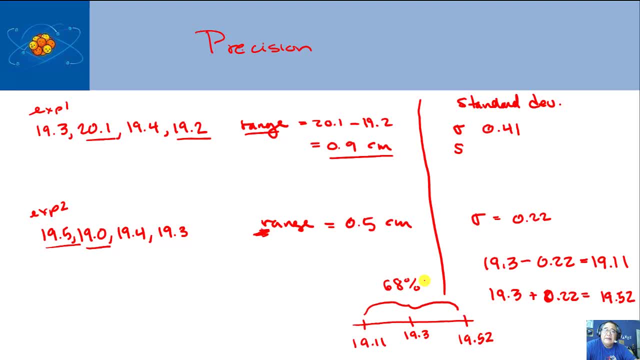 like if it's not strings we're talking about, but we're talking about behavior, like traits of, let's say, an animal's jawline. If you take measurements and calculate averages and standard deviations, you can tell whether or not that that animal's jawline. 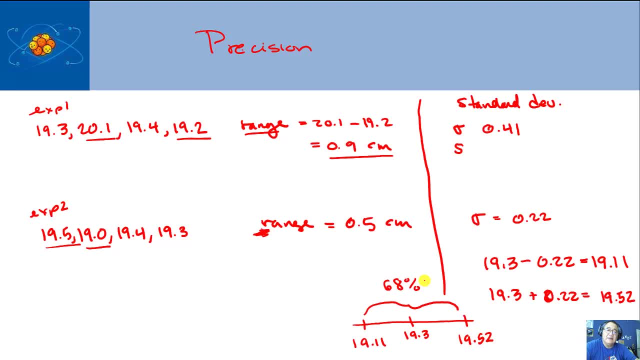 structure fits in with that particular species that you're studying, or maybe that is something different, things like that. Okay, so that's the idea of precision. Again in lab we'll talk about standard deviation a little bit more, but for lecture, for now.